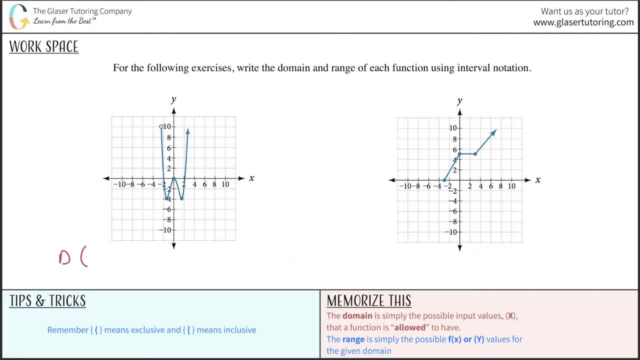 parenthesis, because it means exclusive. So exclusive of all the way from negative 2.5, okay, All the way out. now to: we have to think what's the rightmost portion. Now notice there's an arrow here, which means this graph continues on forever. 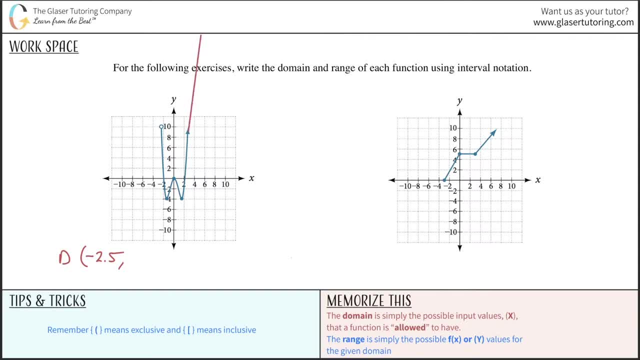 okay, And it's going to be continuing on forever. at a little bit of an angle there, So it's tough to tell, but if you imagine this line continuing on forever, it's going to continue on forever. therefore, in the x direction. 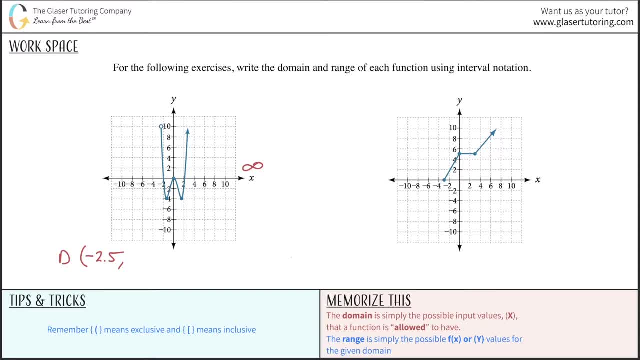 So it goes all the way out to don't know how that happened, goes all the way out to positive infinity, all right. So it goes all the way out to positive infinity, exclusive of it, because you can't actually include infinity. It's not a real number. 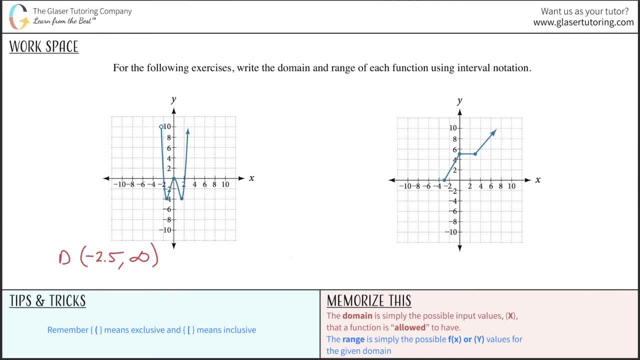 Now, when we think about the range right, We think about the lowest and the highest point. So the lowest point that this graph will reach Is right here at x is equal to negative 4,. okay, Now all of those values are filled in, okay. 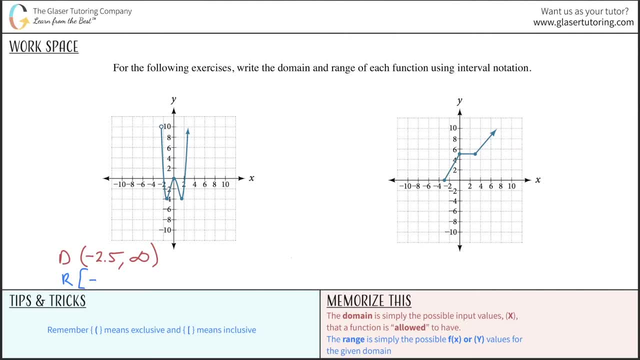 So when we do our range now, it's inclusive of negative 4.. And then what's the highest point that the graph reaches? So don't get confused by this. I don't care what that is, I want to know the highest point. 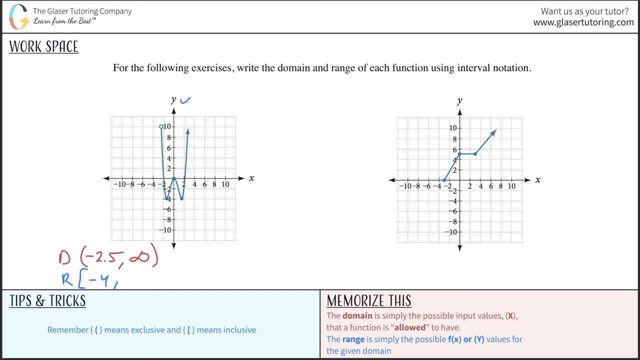 Remember, this continues on forever. okay, So it's going to go all the way up to positive infinity on the y-axis. So therefore, it's going to. that's the upper limit and we can't include infinity because, again, infinity. 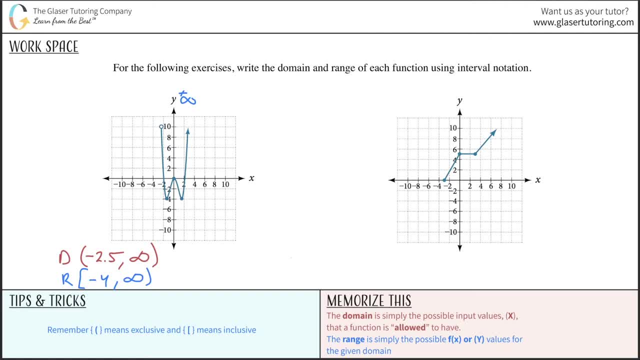 it's infinity, right? I mean, I know that definition is circular, but infinity is not a number, It's an idea, So that takes care of that. Now we can easily approach this right. The leftmost point of the graph in terms of the domain here is going to be right around. it looks like x is equal to. 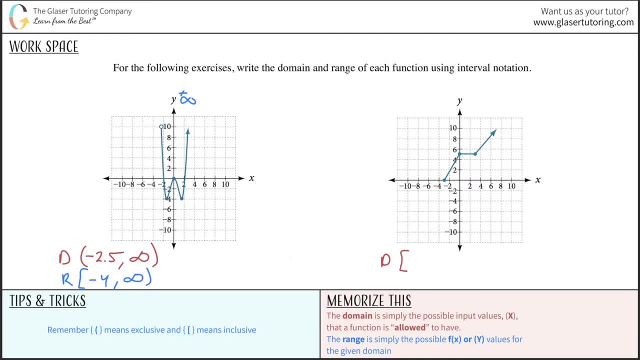 negative 3, inclusive of it, because it is a filled-in circle, So we write negative 3.. Then we have to think: well, what's the rightmost point? Well, this thing is going to go on forever. I don't care that these are filled in, It's just a distraction. I want to know the rightmost point. 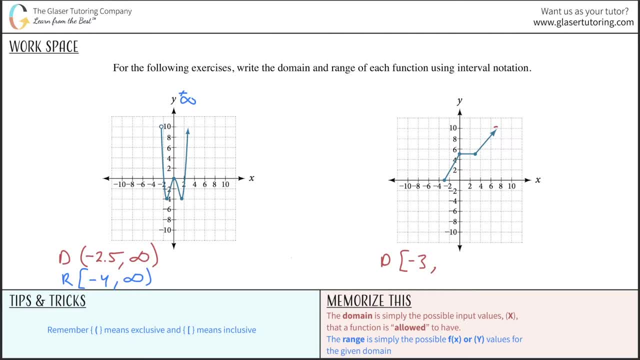 If they were not filled in, then I'd have to worry about it, okay, But if they are filled in, it doesn't matter. They're part of the domain. So, since this is going to continue on forever, it's going to basically continue on forever in the x direction. So therefore, it's going to go.